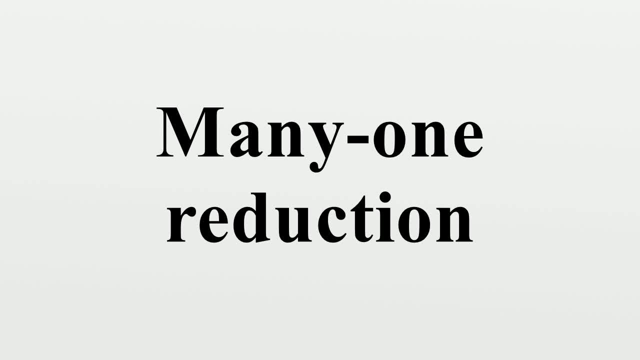 If such a set B is called many-one complete or simply m complete, IFFB is recurrent. Every recursively enumerable and every recursively enumerable set A is m reducible to B. Many-one reductions with resource limitations: Many-one reductions are often subjected to resource restrictions. 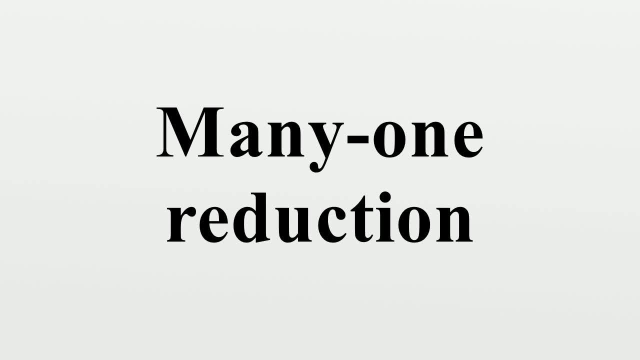 For example, that the reduction function is computable in polynomial time or logarithmic space. See polynomial time reduction and log space reduction for details. Given decision problems A and B in an algorithm N which solves Instances of B, We can use a many-one reduction from A to B to solve instances of A in. 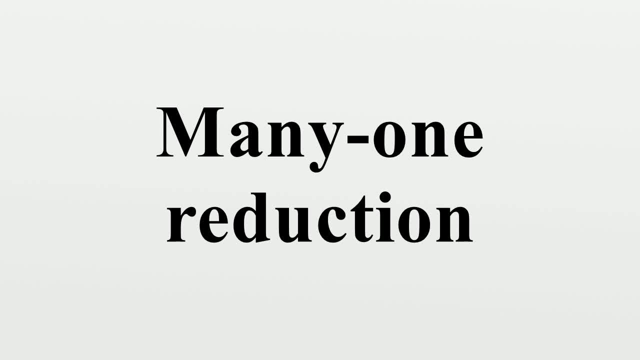 The time needed for N plus the time needed for the reduction, The maximum of the space needed for N and the space needed for the reduction. We say that a class C of languages is closed under many-one reducibility if there exists no reduction from a language in C to a language outside C. 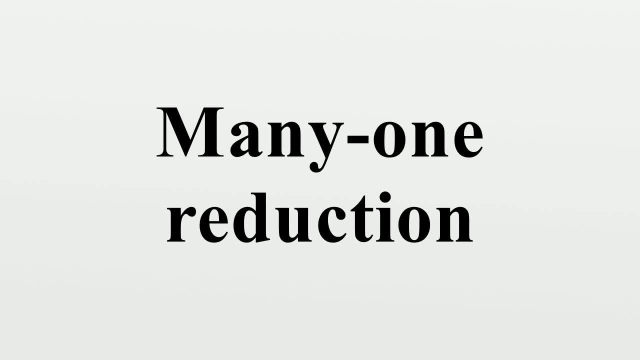 If a class is closed under many-one reducibility, Then many-one reduction can be used to show that a problem is in C by reducing a problem in C to it. Many-one reductions are valuable because most well-studied complexity classes are closed under some type of many-one reducibility, including P, N, P, L, N, I, Co, N, P, P, S, P, A, C, E, X, P and many others. 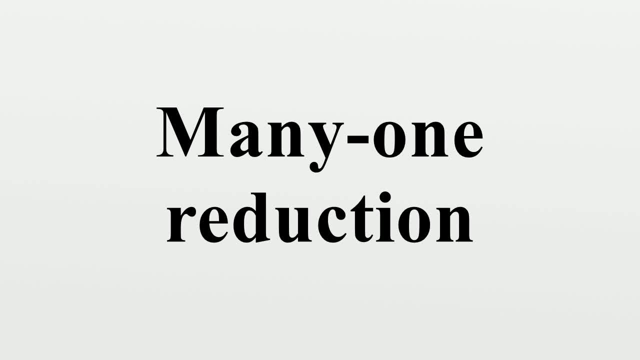 These classes are not closed under arbitrary many-one reductions. However, Properties, The relations of many-one reducibility and one-reducibility are transitive and reflexive and thus induce a preorder on the power set of the natural Numbers. If, and only if, 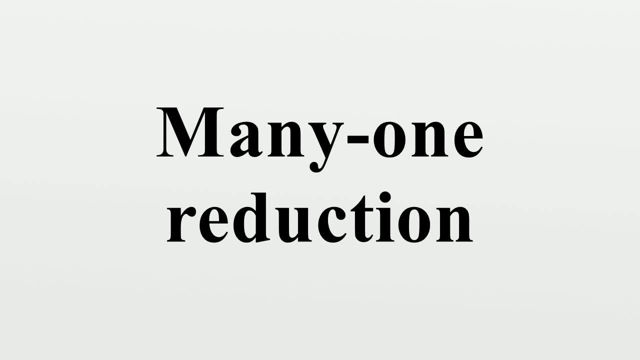 A set is many-one reducible to the halting problem if, and only if, it is recursively enumerable. This says that, with regards to many-one reducibility, the halting problem is the most complicated of all computer programs. Thus, the halting problem is many-one complex.